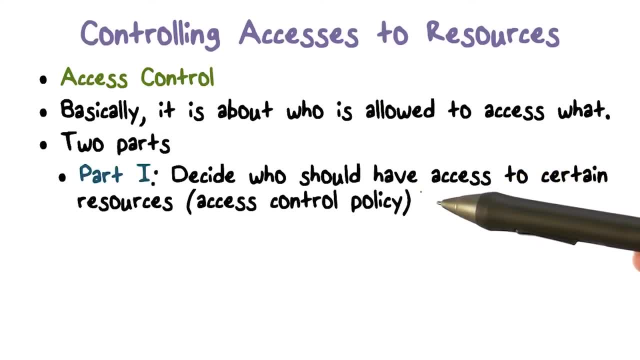 In part one, someone has to specify who has access to what, So this is called an access control policy. So there may be many ways to sort of decide who gets to access what. There has to be a policy we have in place that is going to define this for us. 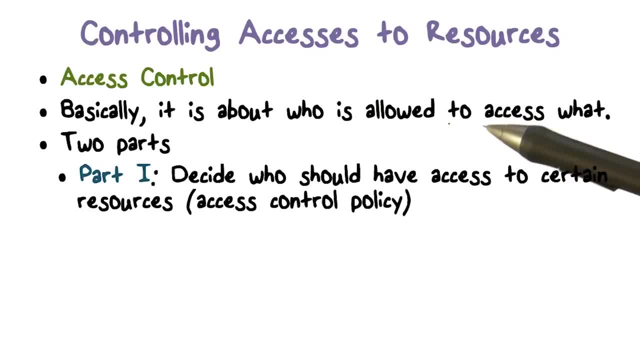 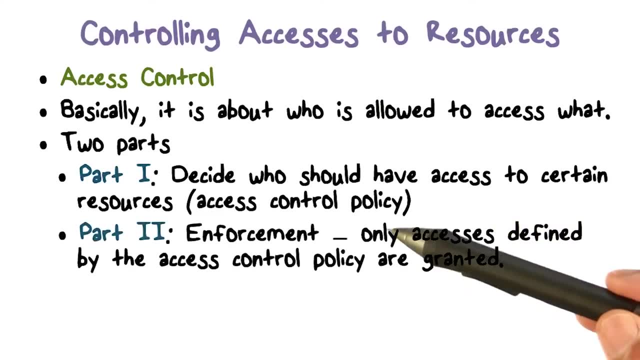 So to answer this question about who can access what is you tell the system how the resources should be shared or who should be given access to what resource. Once you do that, then it's. the part two is about enforcement. The system has to monitor each request for these resources. 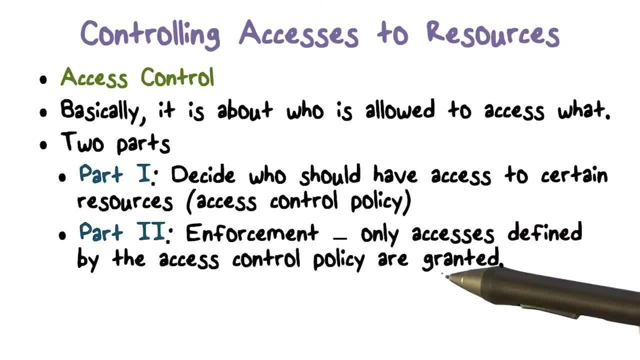 And, based on the policy that tells us who can access what, it should make sure that any accesses that are allowed are consistent with the policy that we have. So enforcement basically says there is no way for you to go and access a resource when that access is not allowed by the policy. 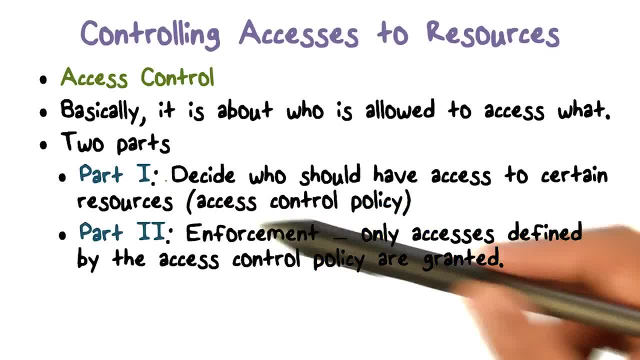 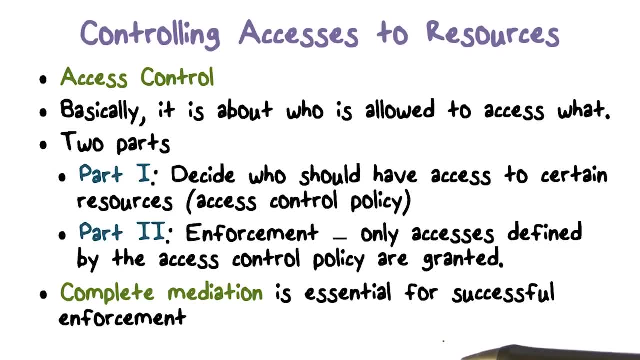 So define the policy that's in part one and then enforce the policy that's part two. Now you can see the importance of complete mediation. Clearly, complete mediation says no one should be able to bypass and get to the resource without going through the trusted computing base. 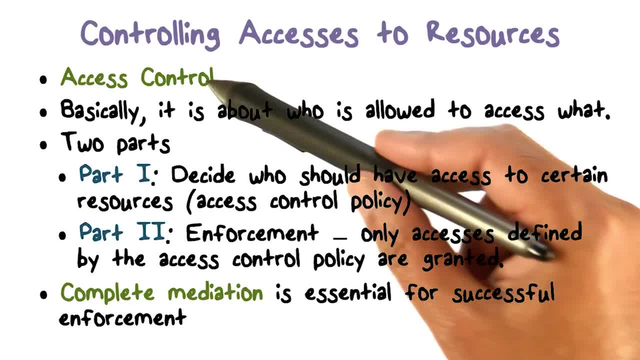 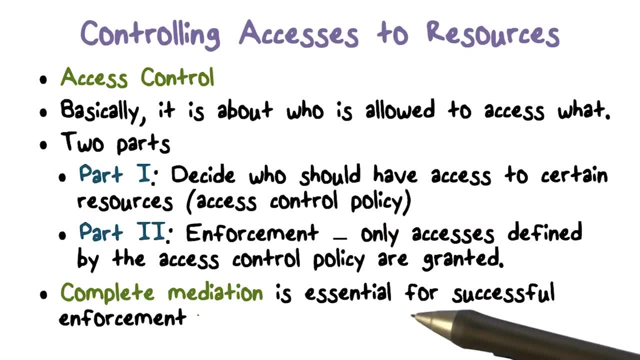 If you don't have complete mediation, we can't perform this check, access control, check that we're talking about. That is possible only when the trusted computing base is involved in a request, and that's why complete mediation is so important. 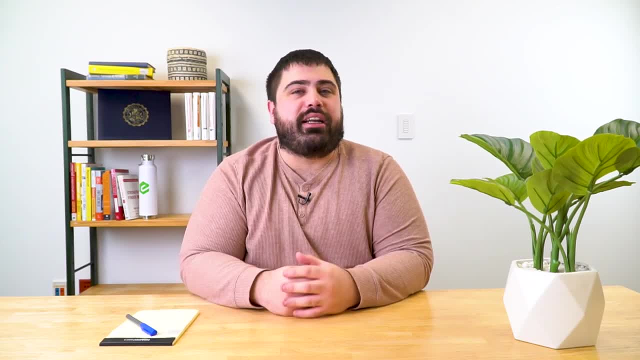 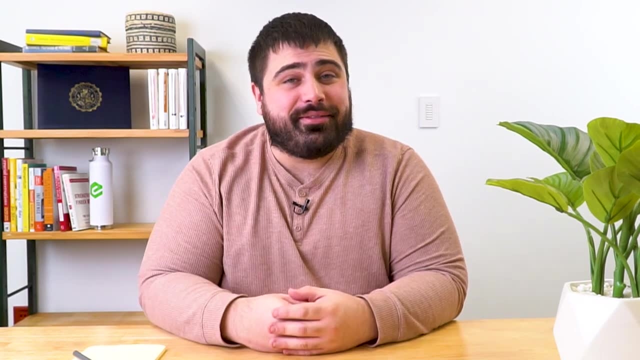 Do you remember work before the internet? We've come so attached to technology that most people can't even fathom what they did during their nine to five before computers became mainstream- I know I can't- From automating internal processes to adopting cloud services. 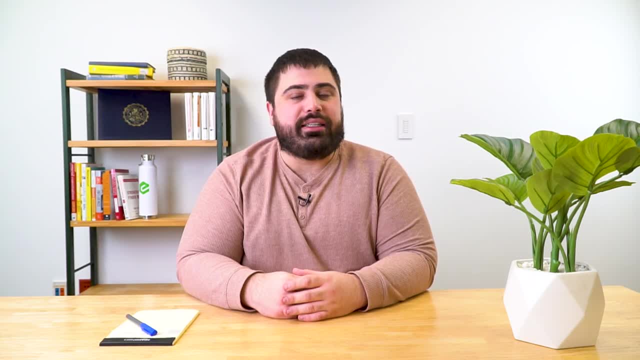 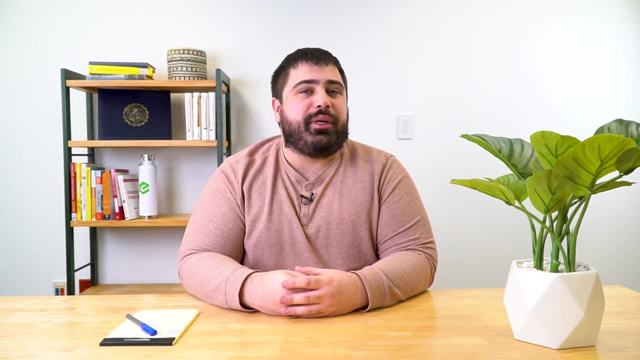 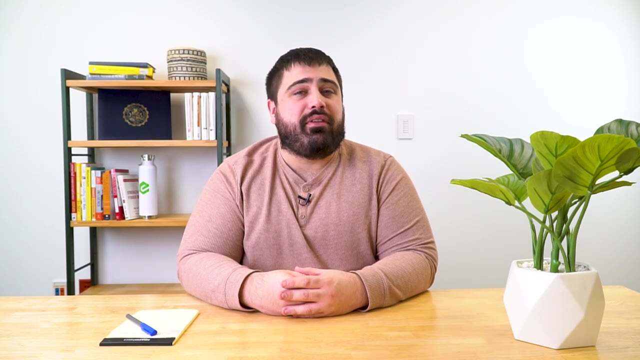 organizations are constantly embracing changes produced by technology. On the other hand, technology poses new challenges and threats to your organization as well. The internet has become an indispensable tool, while also becoming an attractive hunting ground for criminals. Every year, more than 155 million personally identifiable records become exposed. in data breaches in the US alone, And in 2019, the number of cybercrime incidents surpassed 31,000 cases worldwide. In the same year, the global number of data breaches with confirmed data loss rose to almost 4,000.. The average cost of data breaches reaches is your cybersecurity up to par? If you don't know the answer to that question, that's okay. That's why, as an organization, you need to follow cybersecurity risk assessment checklists. Your sensitive data is likely already facing threats and vulnerabilities.